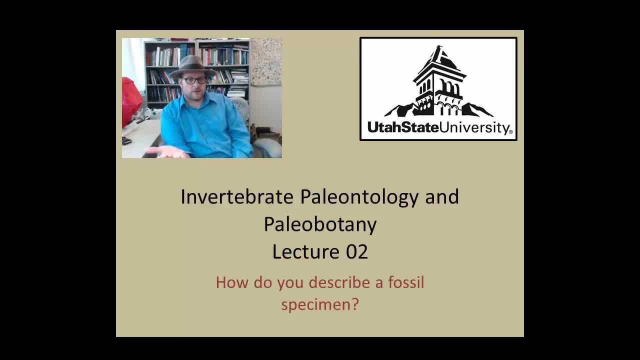 we don't see a change in the fossil record. that's observed, then evolution is disproven. Following modus talonus, we come up with a hypothesis and then we think of ways to disprove that hypothesis. So, following modus talonus, we come up with this hypothesis and then we think of ways. 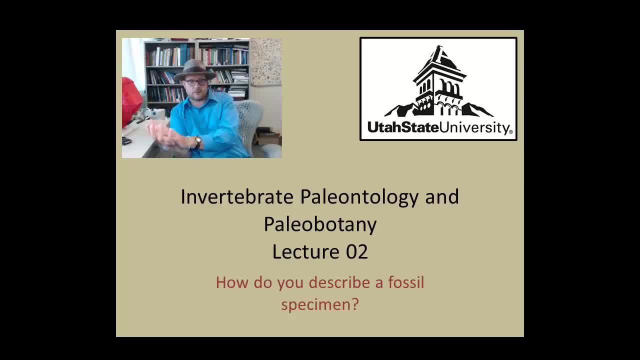 to disprove that hypothesis, And we can do that through a series of tests. Often times you come up with a null hypothesis and then you develop techniques to test that hypothesis. So a hypothesis, then, can only be raised to the level of a theory or principle after many. 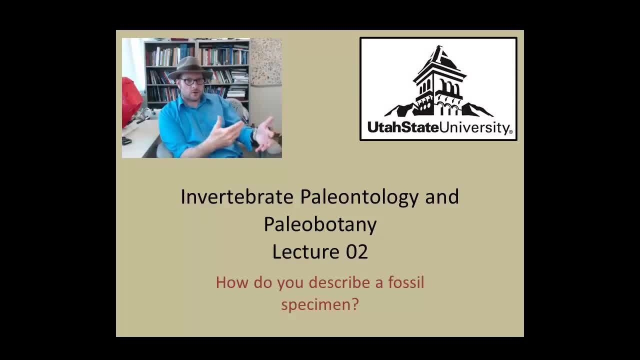 tests have been done that show that we can't disprove it with those tests. So an idea is never in fact accepted, it's always sought to disprove it. However, paleontology sits in the more ancient realm of observational science, A science that is based on making as precise of measurements and descriptions of nature. 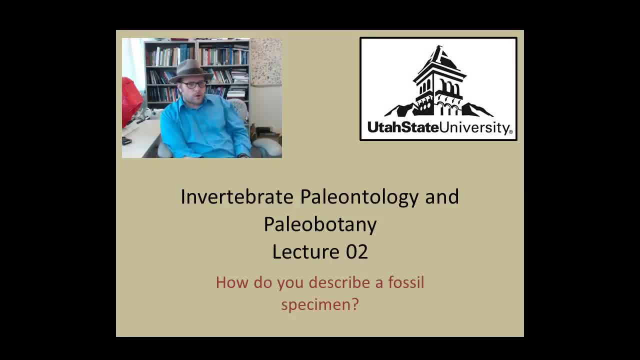 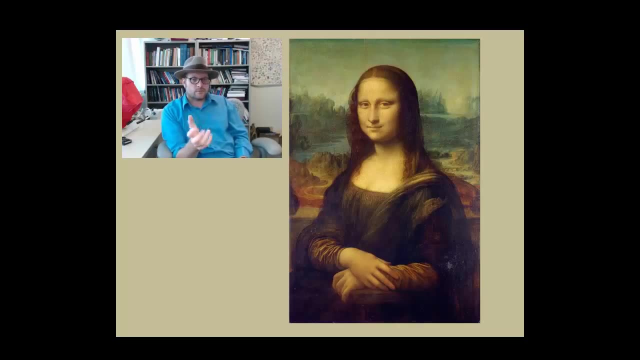 as possible. Paleontology can propose and test hypotheses, but often the science starts with direct observation. This is the science of the Italian Renaissance, where art and science mingled, As people attempted to capture nature as accurately as possible, either in art or in science. 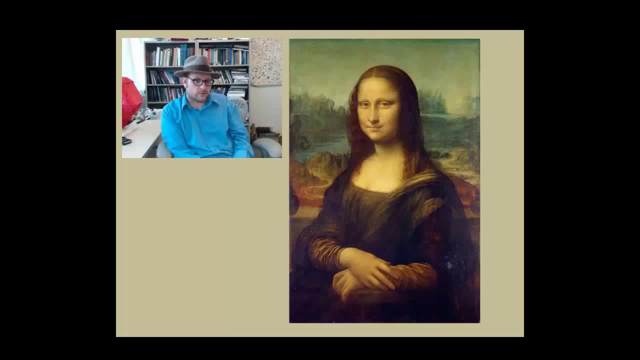 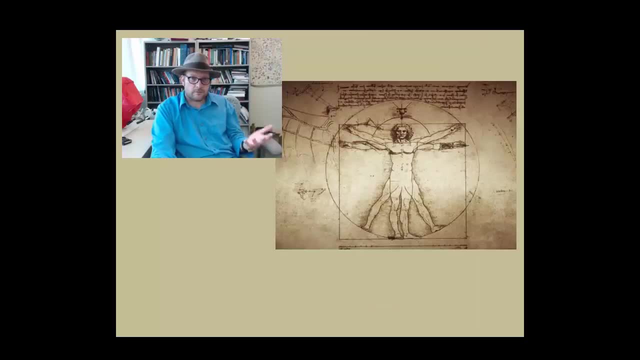 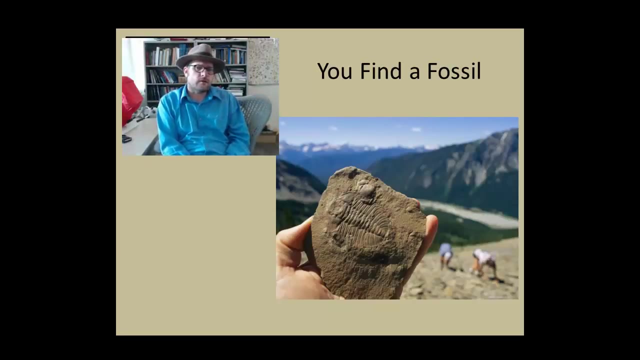 So think of the duality of the Renaissance painters and scientists, where there was little distinction between painting the Mona Lisa and diagramming the human body. The discovery of a fossil is where paleontology begins. We don't question the reality of the fossil, but we set about to uncover how and why the 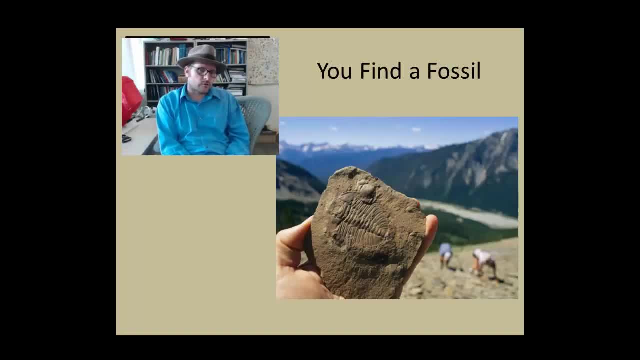 fossil exists, And we do that by describing the fossil in detail and drawing conclusions from the evidence that we gather. However, in describing a fossil, we also must be thinking about the importance of the fossil and the conclusions that we can draw from the fossil itself. 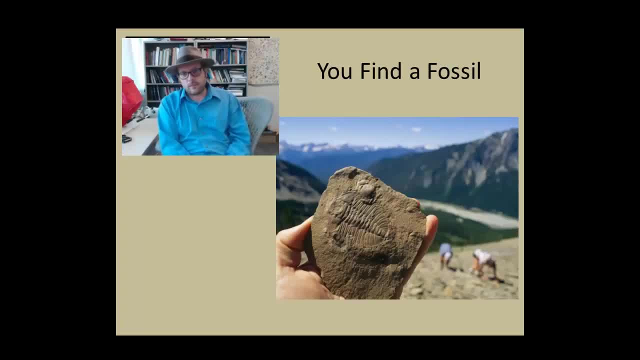 Charles Darwin once stated the following, which I think is a great quote. About 30 years ago he said there was much talk about geologists ought to only observe and not theorize, And I well remember someone saying: at this rate, one man might go into a gravel pit and 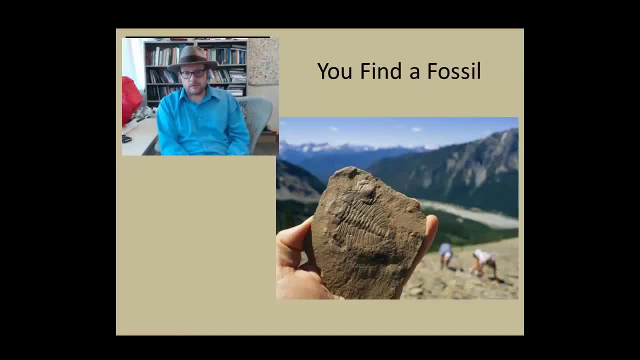 count the pebbles and describe the color of the pebbles, he found How odd it is that anyone should not see that all observations must be for or against some view if it is of any service. So, even though paleontology is an observational science, 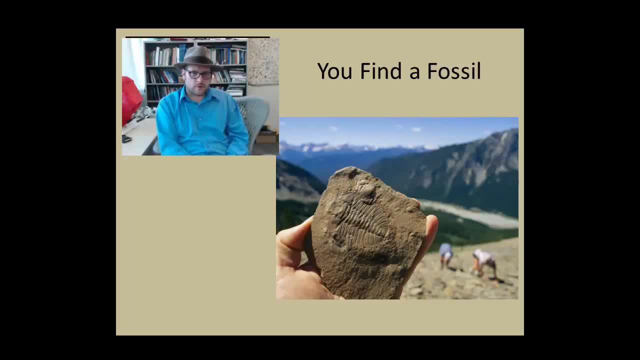 We're talking about the science of the observations of various life forms and not just the physical observations of the objects, mean that it collects the arbitrary, but it sets out to document the unusual, the unique, the missing evidence or the piece of the puzzle to larger questions in science. 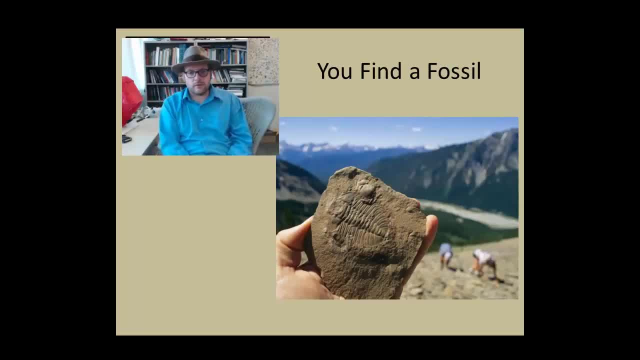 So let's start with a new discovery, a new discovery of a fossil that you've just picked up out in the field. maybe you're looking at a bunch of rocks and you just turn over a rock and see a beautiful fossil such as this trilobite. 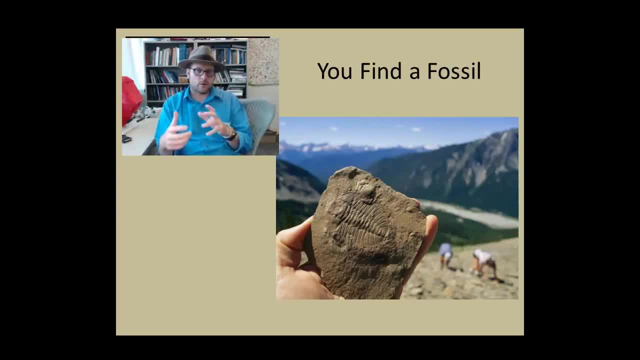 In this lecture I'm going to go over just how you go about describing the fossil, and in the next series of lectures we'll talk more about how you go about identifying the fossil, how to determine if the fossil represents a new species, how you can use the fossil. 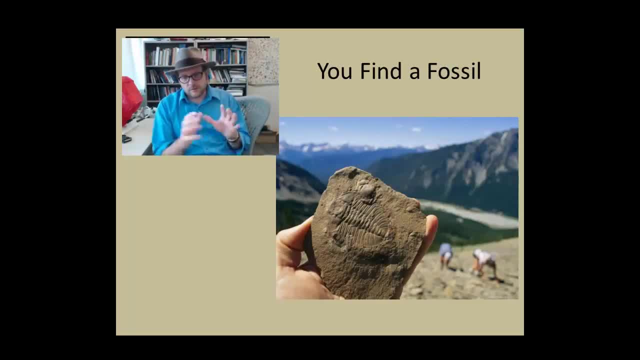 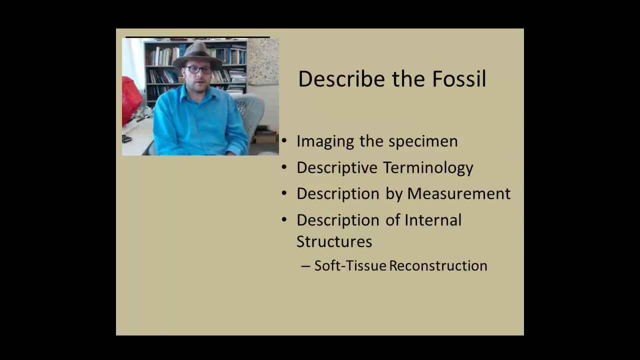 to determine the past environment. So today we're just going to focus our lecture on how you go about describing the fossil. So first we'll talk about imaging the fossil specimen And then we'll talk a little bit about the descriptive terminology you use to describe. 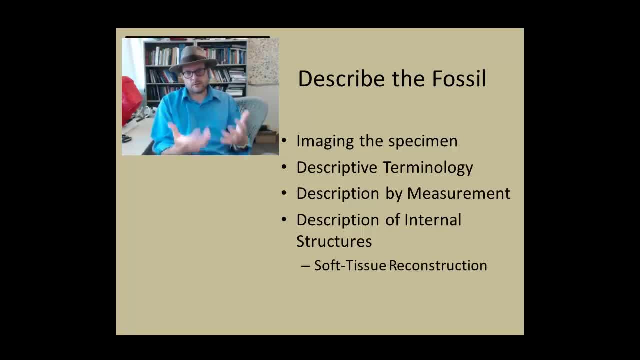 the specimen. We'll talk about how you go about describing a fossil by using measurements. We'll talk about how you can actually get to diagram or reconstruct internal structures And we'll talk a little bit about soft tissue reconstruction. So we're going to really be focusing on sort of the nuts and bolts of how you go about. 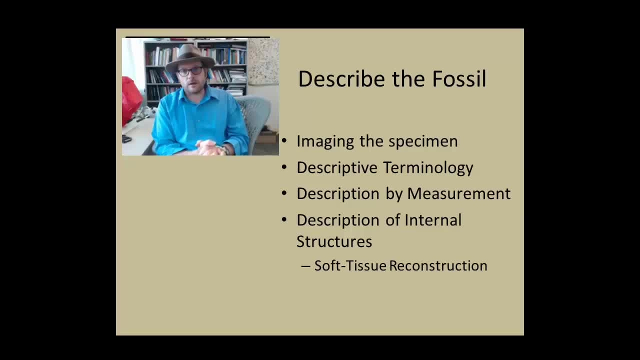 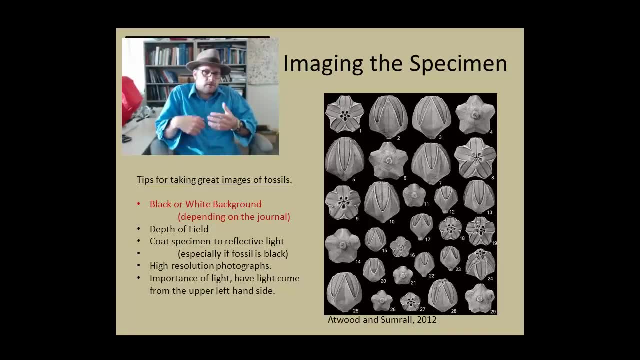 describing a fossil, Maybe one that you have found, Maybe you're working on a research project, So let's talk a little bit about how you go about imaging fossil specimens, And I'm going to give you some tips on things that I've discovered that work really well. 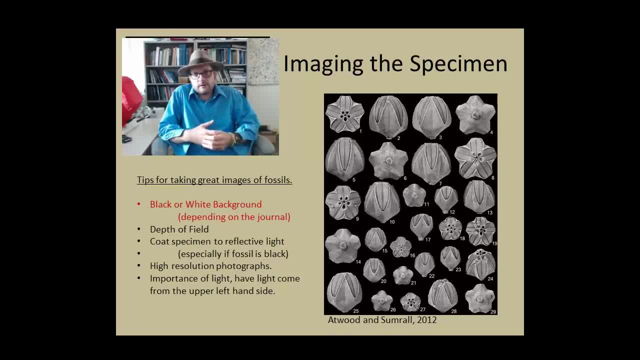 when you set about photographing or documenting a fossil that you've discovered. One of the interesting things is: early on you need to decide if you're going to have a white or black background to your image. So often times to focus on the image. 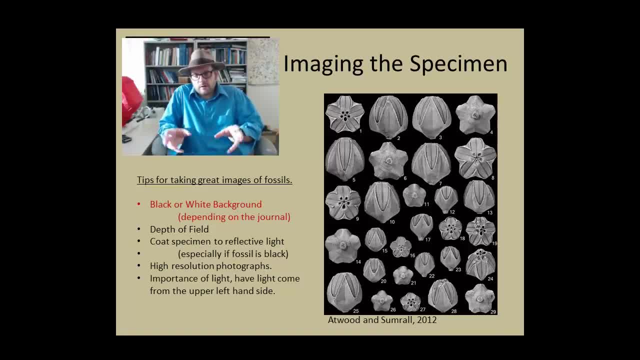 Focus your view on the fossil itself. The outer part. that's not important. the background is often times either converted to black or to white, depending on the constraints of the journal. The journal of paleontology requires a black background, but other journals require a white. 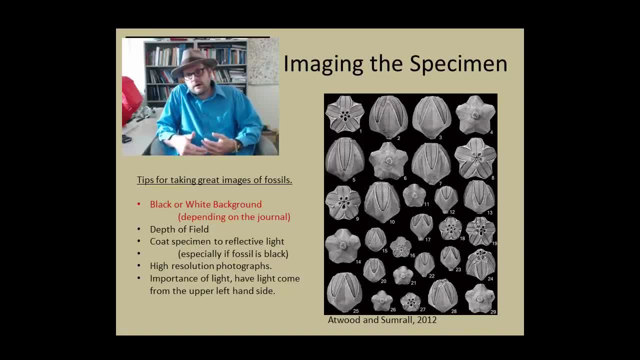 background. Black backgrounds were in the old days of photography. when you photographed a fossil specimen, They had basically overexposed or burned the surroundings. They had basically overexposed or burned the surroundings. They had basically overexposed or burned the surroundings. 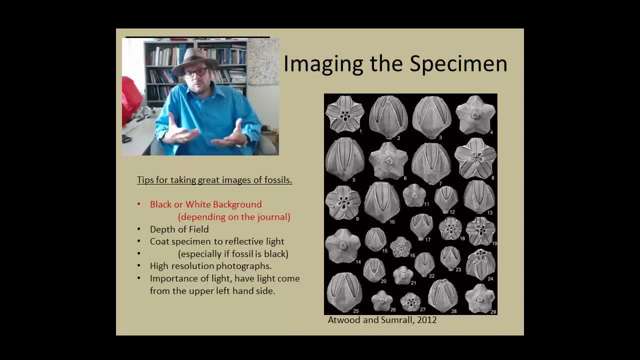 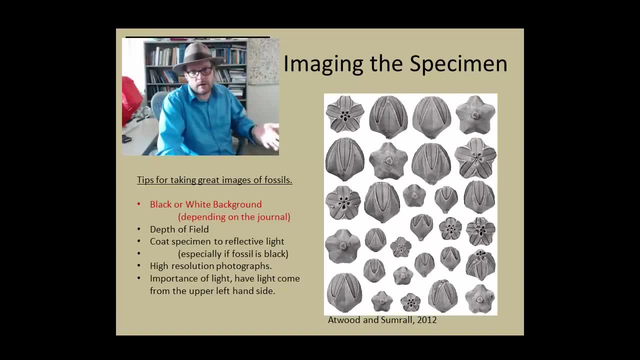 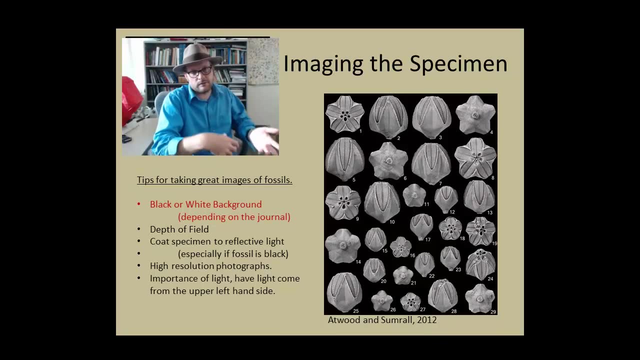 It was a very meticulous process. It was a very meticulous process. Now it's super easy to do it in Photoshop. You can easily put in a layer and quickly go from either a white background, for example in this case, or you can go back to a black background and it's just put in a layer in 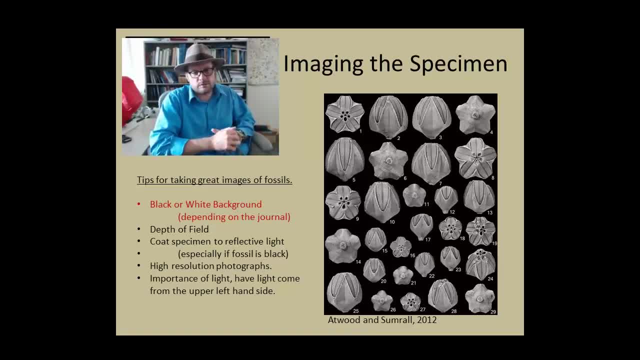 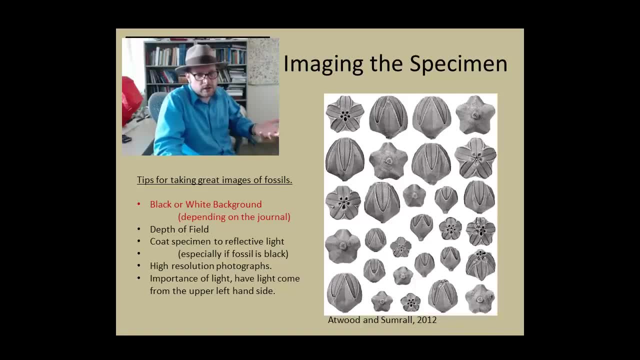 either like Adobe Photoshop or one of the other image processing software applications that are out there. So it's pretty easy to do And you can see how it really changes what you're looking at in terms of these fossils, the types of backgrounds you have. 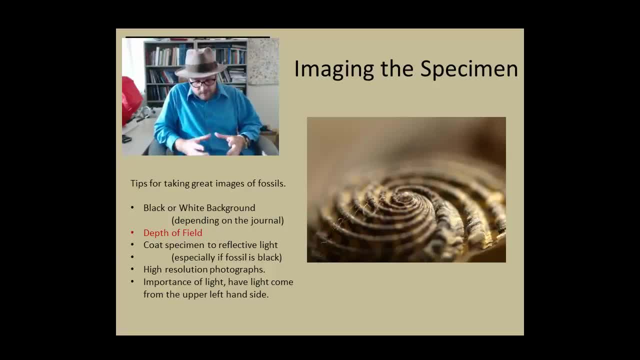 The other thing that you have to be concerned with when you're photographing fossils. oftentimes fossils are pretty small and you have to worry about the depth of field. Many cameras, when you're focusing, will have a limited focus that they focus on. 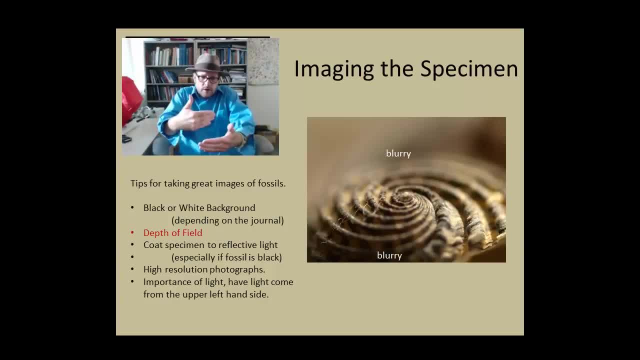 So if you look at this picture here, you can see that in the foreground it gets blurry and in the background it's blurry and there's kind of a middle zone there where the lens is in focus. You often have this problem when you work in microscopes, where you have something that 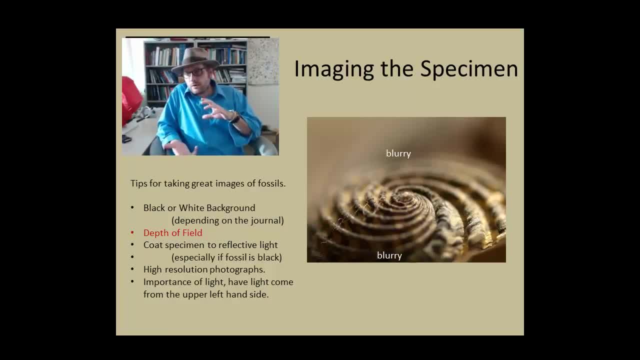 projects out into the space. This can happen with really big specimens as well. If you're trying to photograph, say, a big skull of a dinosaur or something like that, there'll be portions of it that are in focus And portions of it that are out of focus. 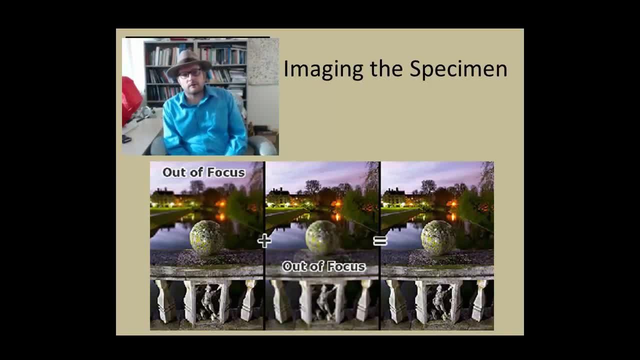 So you have to figure out a way to deal with this, And one of the ways that a lot of paleontologists deal with photography is to take numerous pictures and just change the focal depth. So here's an example where you have the foreground in focus and the background's out of focus. 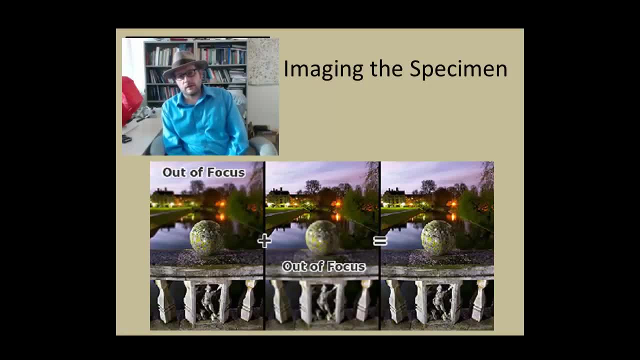 You then take that picture. you take the same picture, but now you have the background in focus. You take the background in focus and the foreground out of focus, and then you take those two images and you stitch them together in Photoshop as different layers and you use the background. 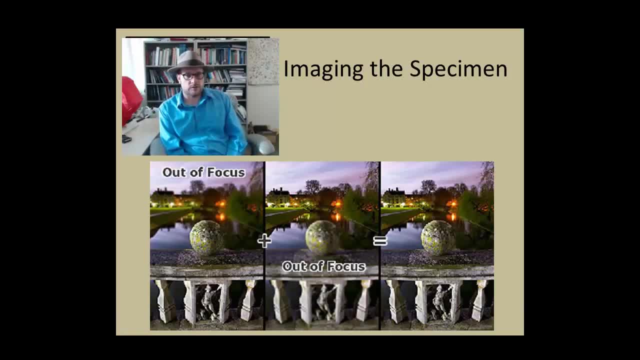 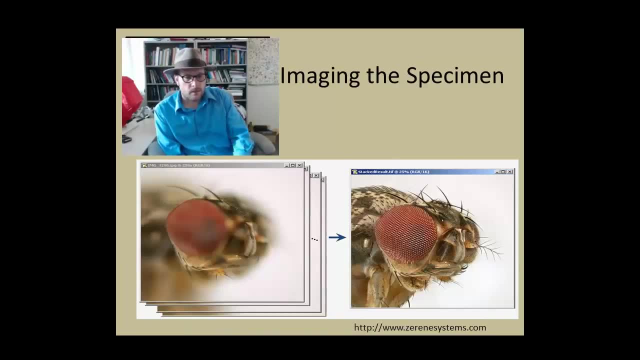 that's in focus and the foreground that's in focus, and you get a nice sharp image. And this is one of the ways you can do it manually, oftentimes using Photoshop and doing a number of layers. Nowadays there's a number of software applications that allow you to do this, especially if you're 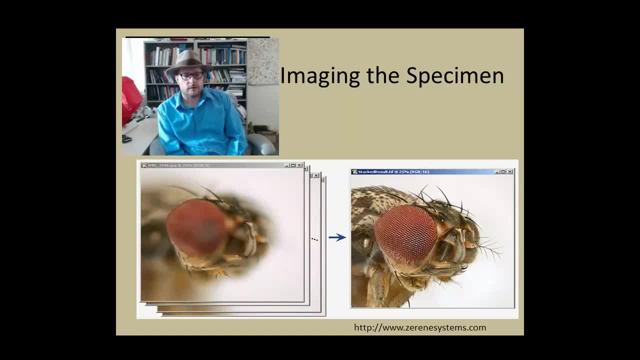 photographing things through a stereo microscope. There's software applications that allow you to stack these images very quickly. What the software does is it basically you run through a bunch of focal depths, so you just change the focus of the microscope to go through all of those different layers. 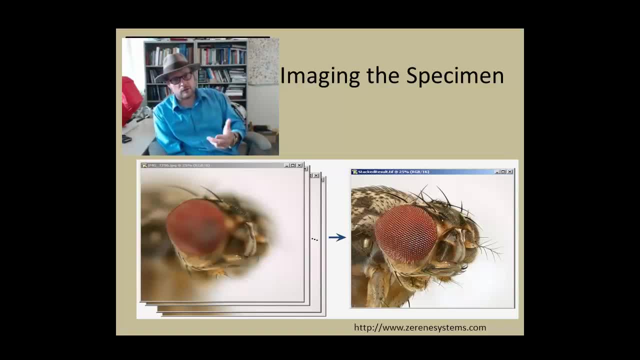 And so you go from the bottom to the top, make sure everything's in focus, And then you can enter it into some software that'll go through and it'll stack those, And so the software will identify parts that are in focus and parts that are out of focus. 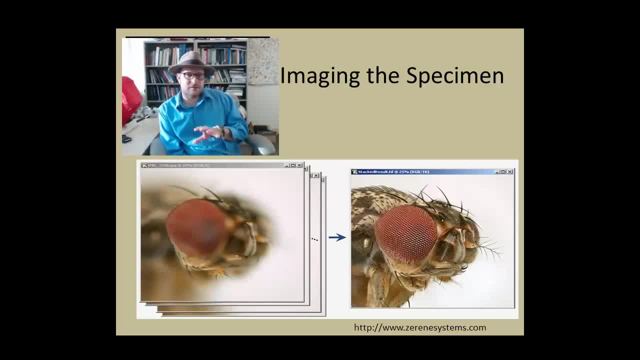 and allow you to stack the image, And so the entire image is in focus, and you can see that with this example of the head of a fly. So photographing really small specimens like this produce these really incredible images. So each of those layers is in focus and you can take now- usually it's like 20 images. 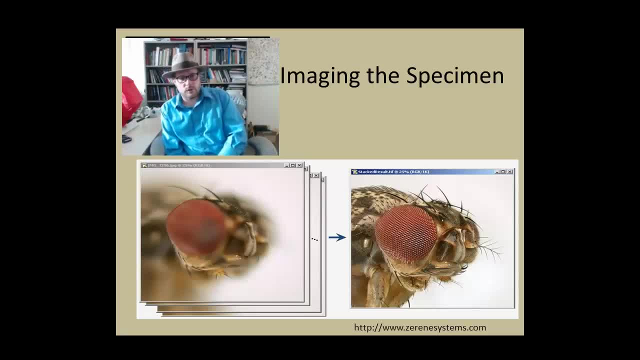 and you can stack those very quickly. The one thing you have to be careful of is when you do that focal change going through. you can't adjust or move anything, So everything has to be still as you're going through those focal things, because if it, 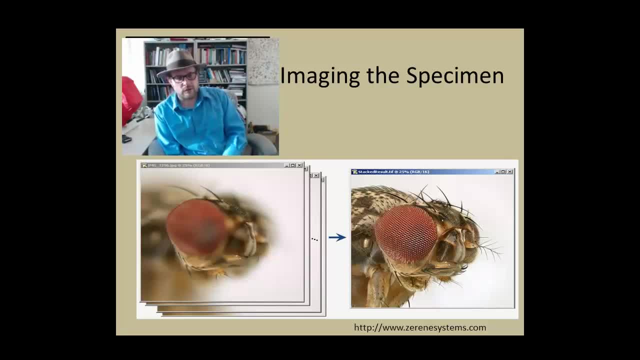 shifts or change positions, it'll just create a blurry image. So that's one of the tricks to do it. So you can do it manually using Photoshop, various stacks, or you can use some of these software applications, And they're getting better at being able to produce some really nice images. 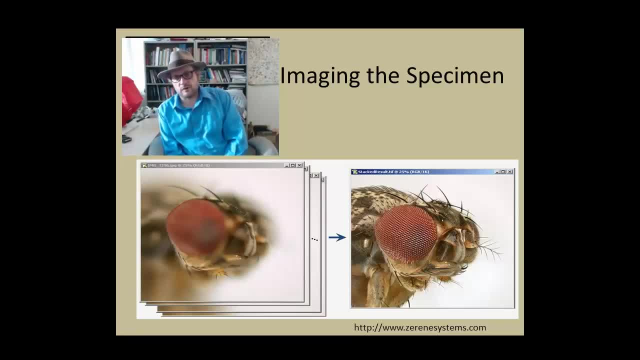 You can actually use these to get stereo images, and that is that you can get ones that are just corrected, just enough that you can actually get a 3D image If you stare at the two different pictures, and you can do that for publications as well. 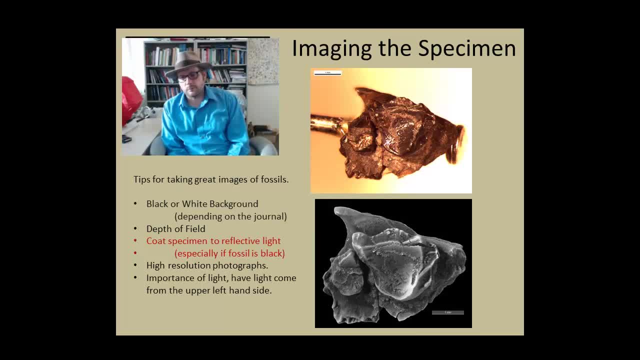 One of the biggest challenges, I think, with paleontology and photographing specimens is dealing with the nature of the fossil that you're describing. This is an example from one of my research papers and this is a little mammal jaw fossil. You can see it's really small. 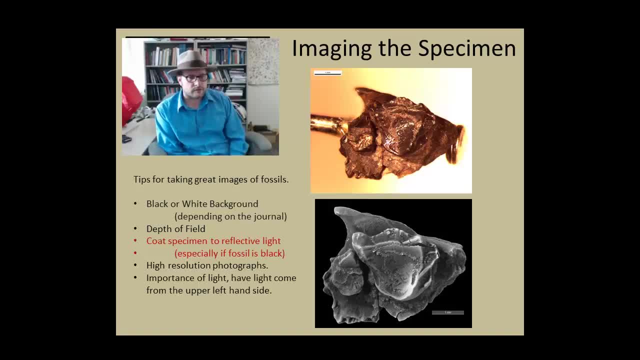 It's a head of a pin there, So it's very, very teeny. It's a teeny fossil. That scale bar is one millimeter. So the problem I have is that if you photograph this just through a microscope, you get a. 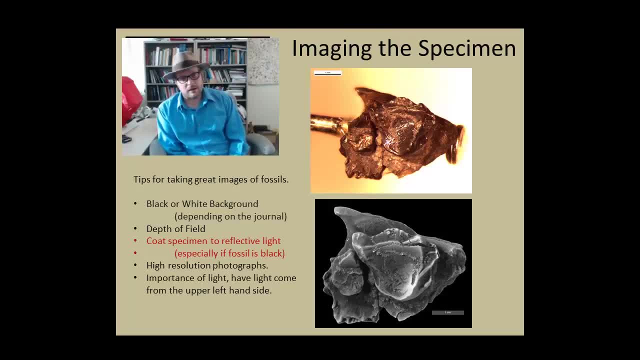 lot of reflection And because the fossil is black and a lot of fossils are black, it tends to basically absorb any of the light that you shine on it And then it tends to be kind of shiny, so you get that shiny part that flashes back. 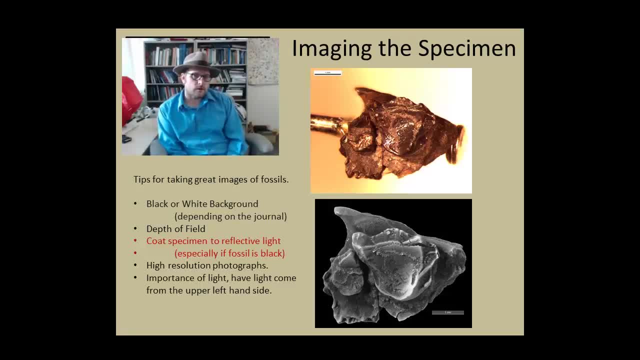 So you can't see the real detail of the specimen. So what paleontologists tend to do is they take the specimen And they coat it in some sort of white powder of some sort, so that when the photograph is taken it basically reflects that light back into the camera lens. 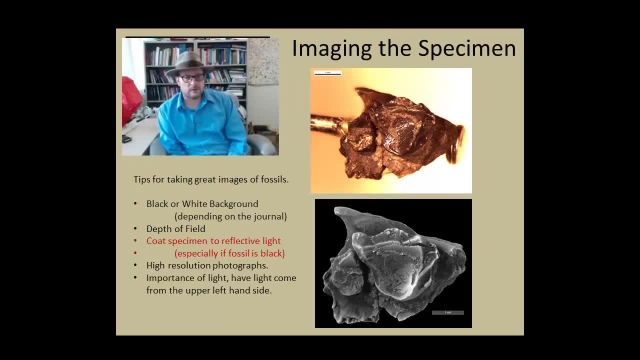 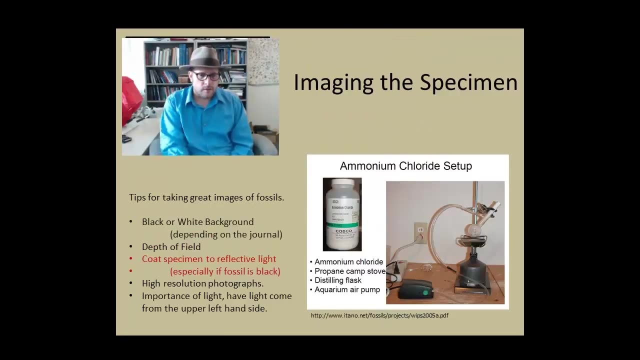 And you get a cleaner picture image of that fossil. So you can see the top image is one that I didn't cover and just used a microscope to photograph And the bottom one is the specimen where I've coated it in a white coating And then photographed it. 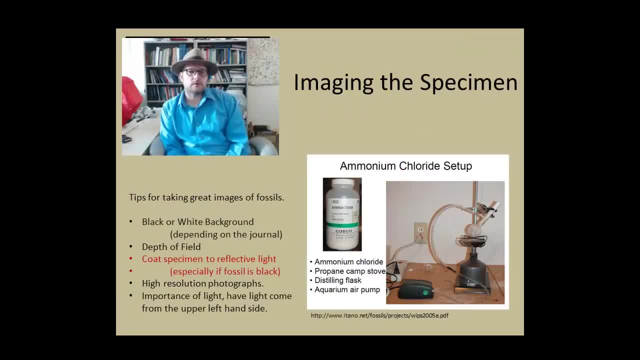 There's different ways to apply this coating. If you're dealing with a bigger specimen, this might be a better set up, And that's using ammonia chloride. Ammonia chloride: you put into a vial And then you can heat it up over a burner. 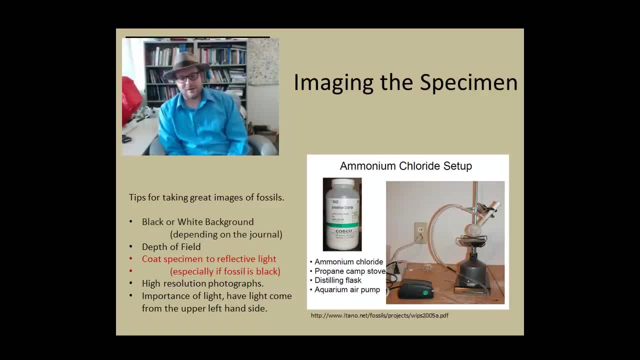 And that produces this white powder that comes out. You want to do this under a film hood so that white powder that comes out you don't breathe it in Because ammonia chloride is poisonous. Another technique that I use if you're dealing with smaller specimens is using magnesium. 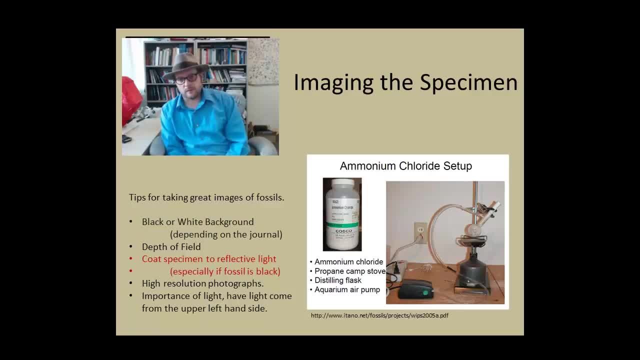 strips And you can take a match and light it And it produces a smoke. that's magnesium oxide, which is very white, And you can quickly cover the specimen. Now this white coating on the specimen can be wiped off. It just kind of lightly dusts the specimen. 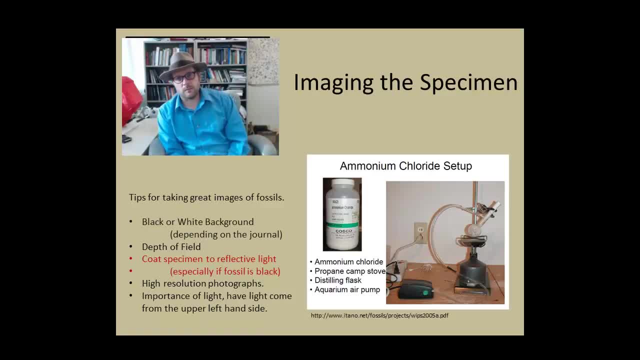 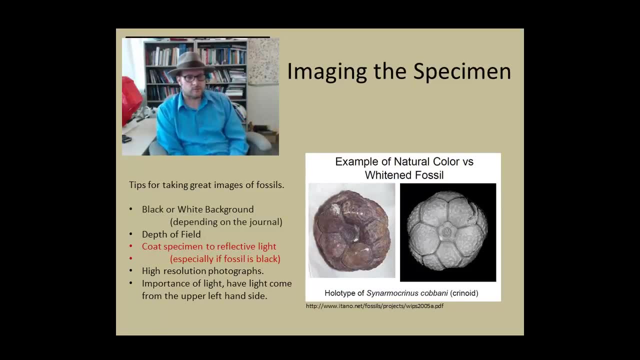 And you don't want to put too much on it, Because if you put too much it'll start to glob up And it'll obscure any of the features that you want to highlight. So here's kind of another example of a specimen, just photographed without a white coating. 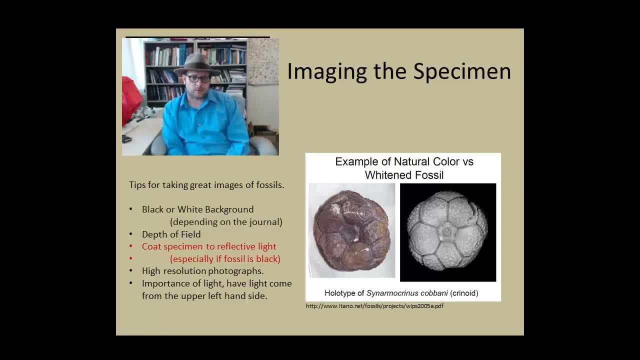 And then, with the whiting added to the specimen, Here's an invertebrate. So one of the really neat things about this is that you can actually reveal a lot of features in the fossil that you wouldn't necessarily have revealed if you just photographed it. 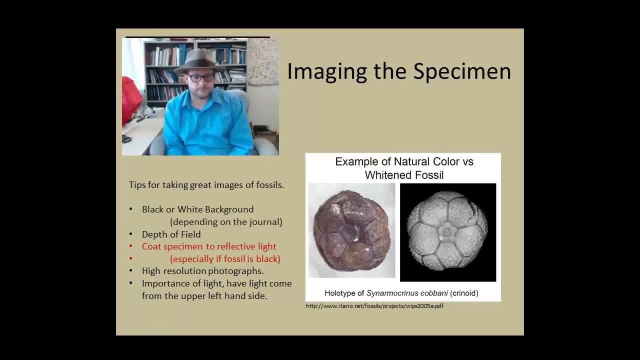 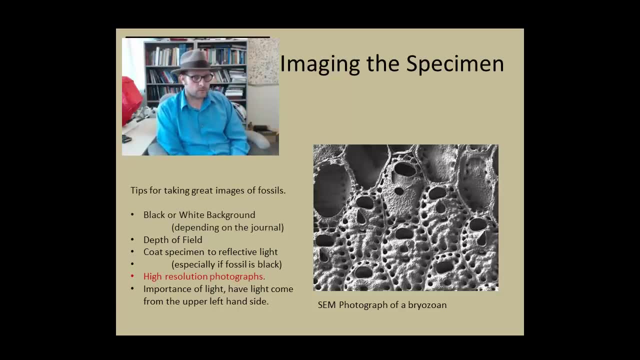 straight, So it's a great technique And it's easy and inexpensive to do. One of the other things you can think about doing is high resolution photographs, And when we talk about high resolution photographs, we can talk about really big, large files. 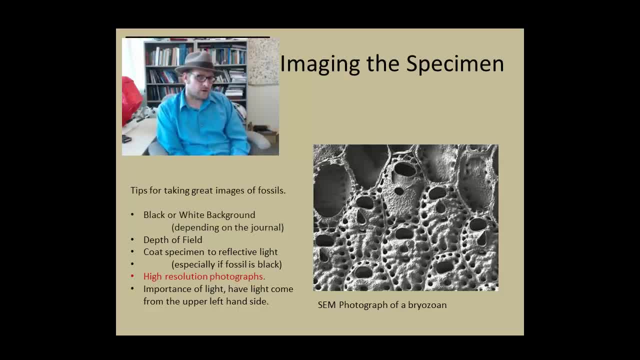 But mostly what we're talking about is using SEM photography. So SEM stands for Scanning Electron Microscope. So SEM is a specialized microscope that basically can photograph a specimen, And they're really good for specimens that are below about five millimeters, although 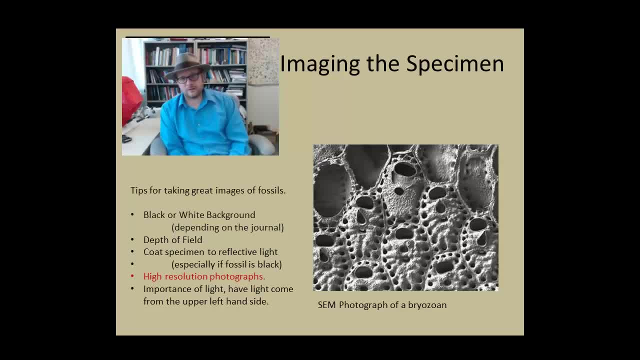 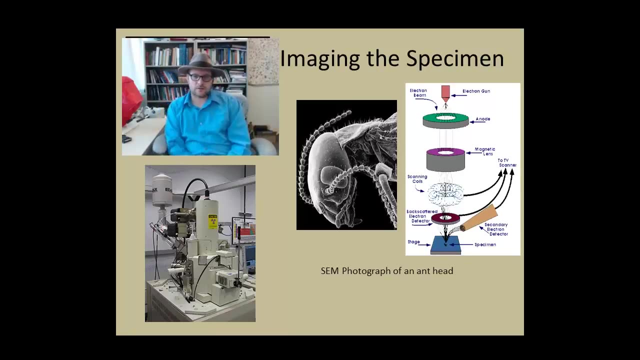 I've seen larger specimens up to like 15 or 20 millimeters, So that's like two or three centimeters is kind of the maximum size. You have to kind of stitch the images together. Now, how SEM basically works is that an electron beam shoots out little electrons and electrons. 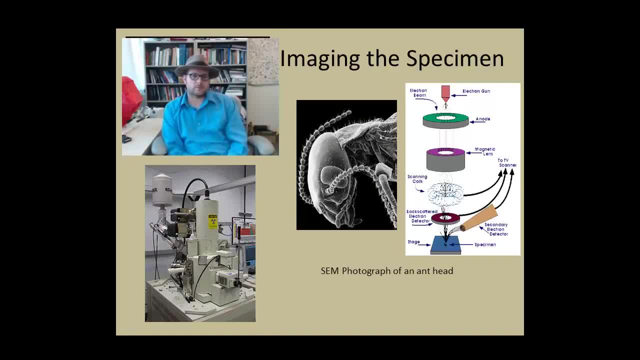 go down through, They are focused onto the specimen And then they bounce off the specimen And then those electrons are picked up by a detector And using that detector they can reconstruct where those electrons bounced off. So it's not light, It's actually these electrons. 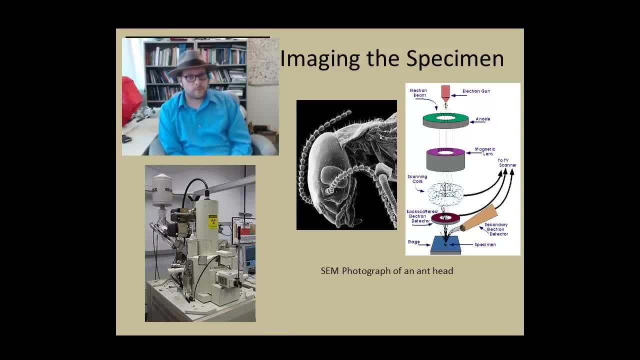 So you can go at a very, very small scale. There's a couple problems with scanning electron microscopes. In the old days, in the older scanning electron microscopes, you had to coat everything in gold, And the reason for that was that the gold would basically 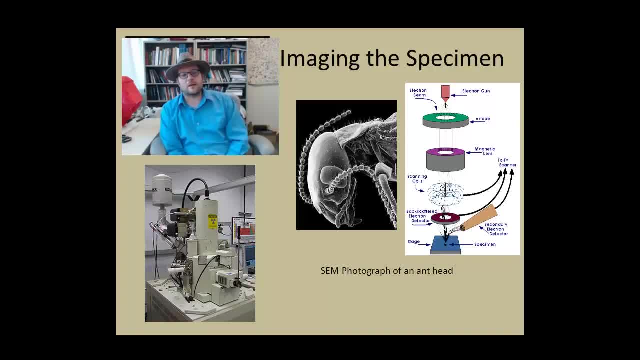 bounce off the electron. that's a metal. The problem was is that a lot of museums didn't want this gold applied to these teeny little specimens And it's kind of expensive, It's a pain, It's kind of destructive to the fossil. 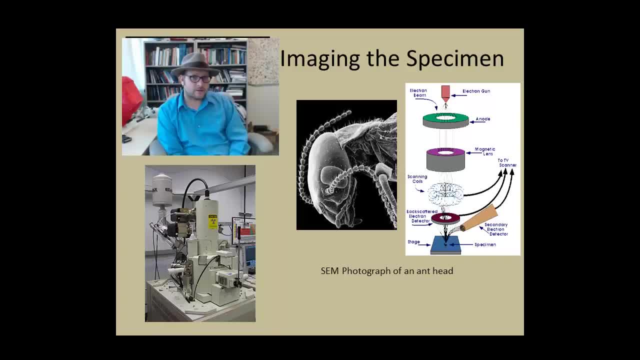 Nowadays, a lot of SEMs are what are called environmental SEMs, And they allow you to do SEMs on specimens that don't have a coating, And a lot of this was developed with a program. It's called the SEM. It's called the SEM. 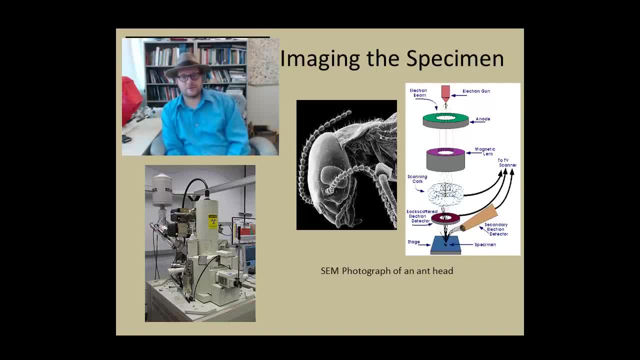 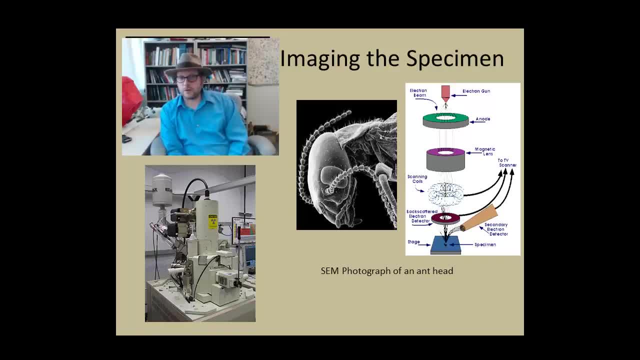 a gold coating. So they use these environmental SEMs And they do pretty good. The quality is not as high as the gold plated ones, but they're really good. And here at USU we have a new SEM laboratory where we can do some of these SEM images. 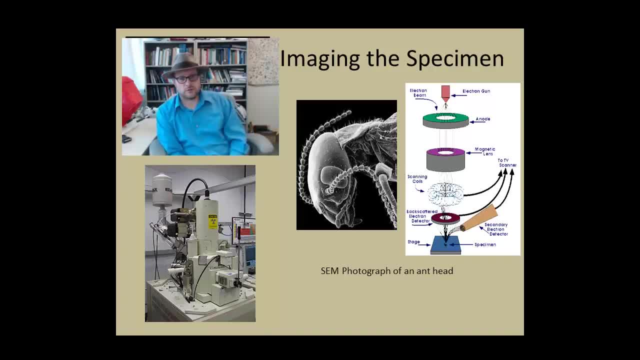 It's a big process doing one of these images- a huge tube. it's not like a traditional microscope that you can look through a lens. you actually put it into a platform, shoot the electrons at it and then the screen pops up: your specimen. 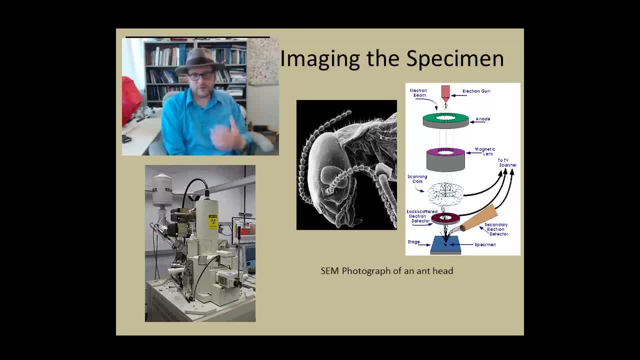 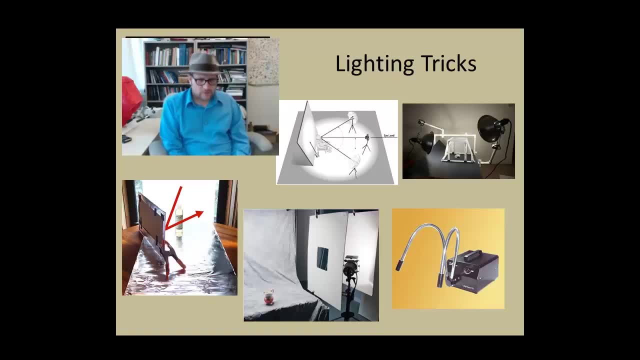 whether you got it or not. So it's kind of a new tool and it produces fantastic, wonderful, wonderful images of these things. So one of the things you need to worry about lighting the fossil properly. one of the biggest problems you have is that: getting light to go into all the cracks and crevices of the 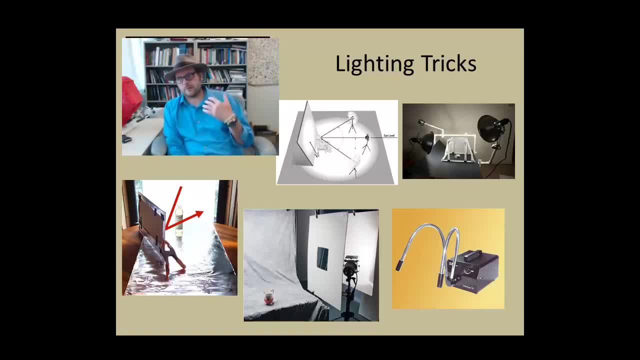 fossil that you're trying to photograph. Often times, one of the biggest problems with fossils, I think, is they're not very photogenic, And so sitting down and really spending time directing your lights is really important. So there's different ways you can set up a studio to photograph your fossils, and that 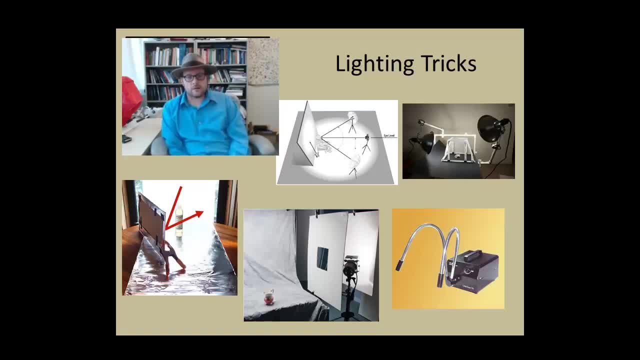 is to have a number of different light sources. Another thing that you can use is aluminum foil to basically put that aluminum foil in certain places that you want to highlight in the fossil, And so this way you can get into those cracks and crevices of the fossil to photograph. 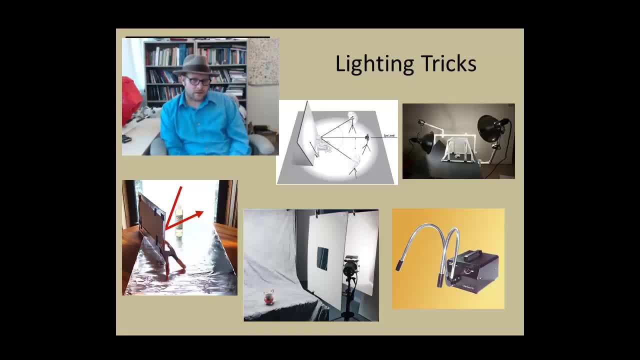 and spend a lot of time playing around with the lighting, taking lots of different pictures at different orientations and spending a lot of time. One of the really nice things you can do is invest in one of these flexible sort of light light projections on here, but it basically will have little lights that you can really. 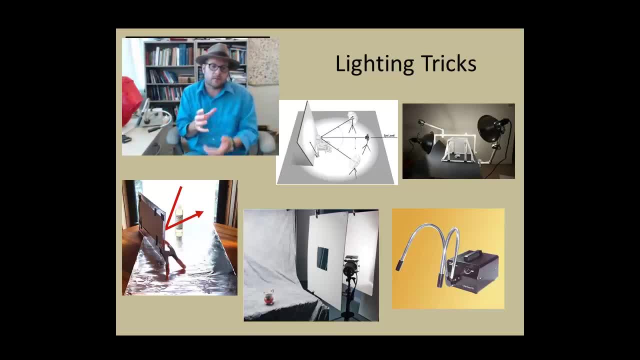 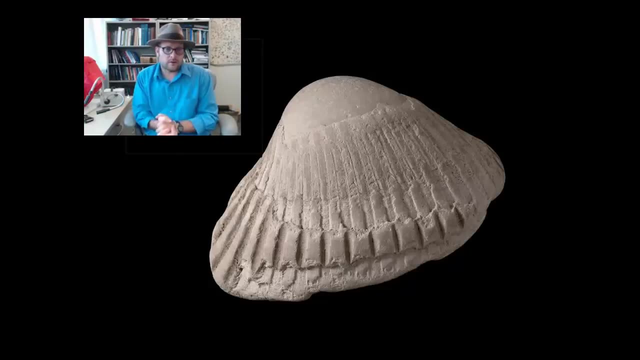 put around a fossil and spend some time directing the light in certain places. So these little lamps are really helpful for doing that sort of stuff. So spend time with light and I want to show you a really good specimen with some excellent lighting. Here is a fossil. 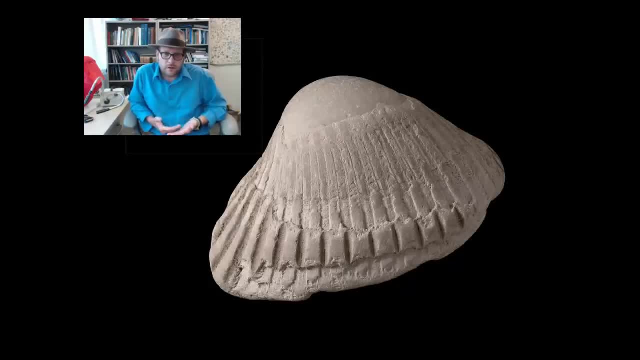 This is a fossil shell where we have excellent light applied to the fossil. You can see that none of the fossil is in shadow or in darkness, so you don't see a really strong contrast. You can make out the features from one side of the specimen to another side of the specimen. 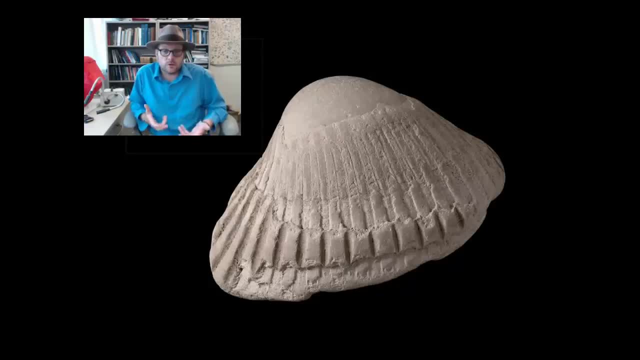 You can see that the entire specimen is in focus, And so this is a really good image that you can use for a publication and really share with other scientists. So this is the type of image that you want to do. The one downside to this image: 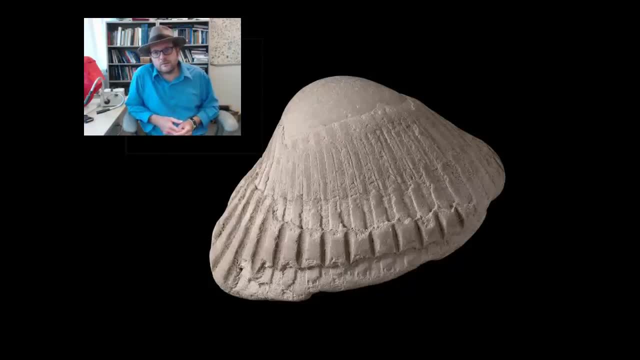 This image doesn't have a scale bar, and so one of the things you oftentimes want to put into an image that you're taking of a particular fossil specimen is a scale bar, And then you can send this to lots of people and share this information, and it's very 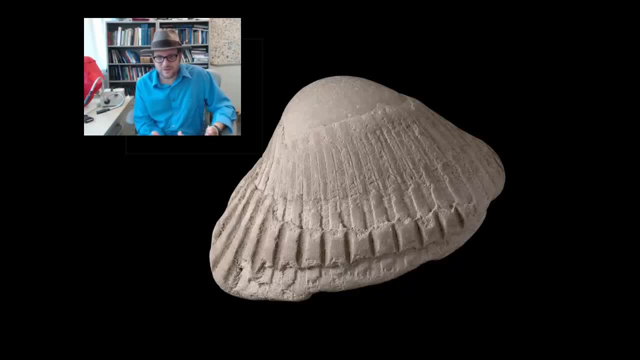 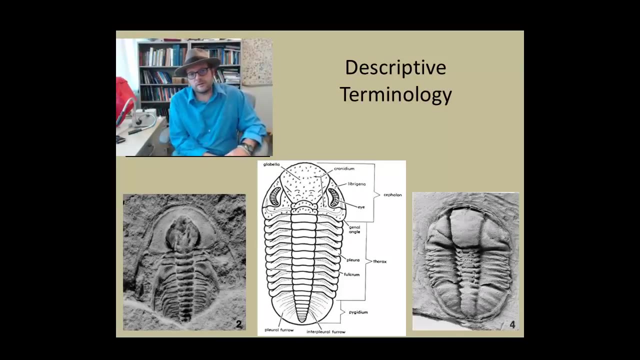 important because it really shows and captures the specimen. It's not out of focus, It's not in shadow, It's just a really good image that you take. So, besides taking images, one of the important things is to learn the terminology of the. 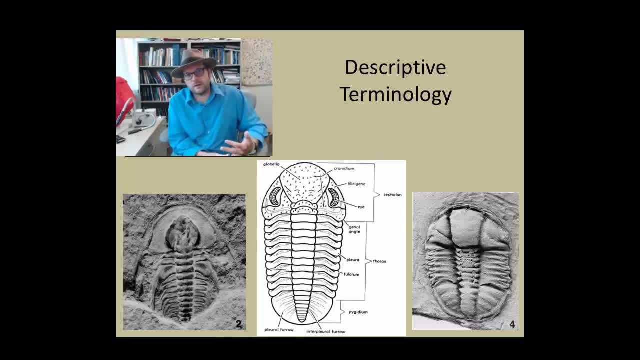 fossil specimens that you're working with Throughout this semester. we're going to be talking about a lot of arcane terminology that's used for various fossil groups. Here I have some trilobites, for example, and so we're going to learn about what Ecabela. 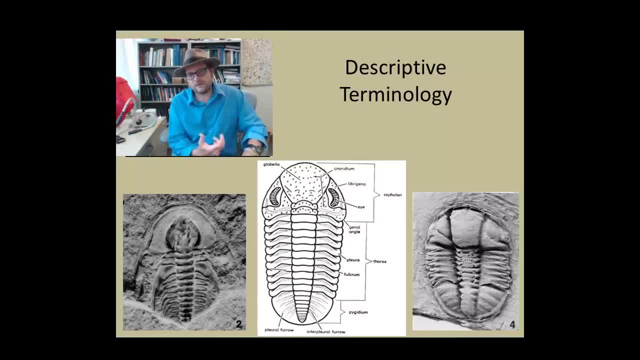 is, And so you can use that in describing fossils, And one of the things that you discover is, as you go into a particular group of fossils, you have to learn all this new terminology. The terminology is really important, Because without this terminology, people might call it the nose or the eyes or the stomach. 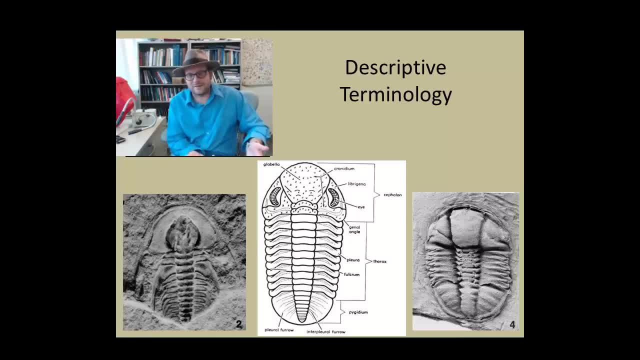 People call it different things, trying to equate it to humans, and none of it makes any sense, so they need to come up with new terms. This drives students crazy, because there are hundreds and thousands of new terms to use in describing fossils. 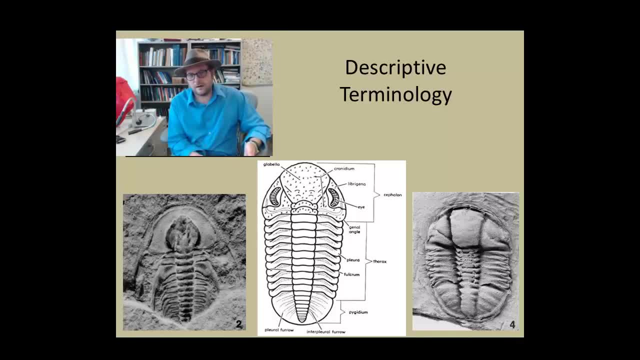 You just have to learn these terms. but once you learn them, then you can communicate with other scientists very effectively. They know what you mean when you say the Gabella is very large or very small. They know exactly what you mean and so you develop a language to communicate with other. 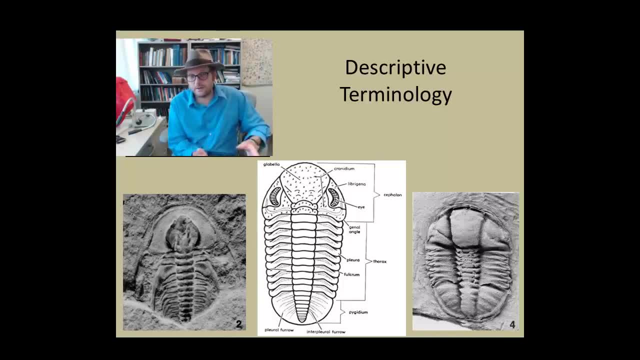 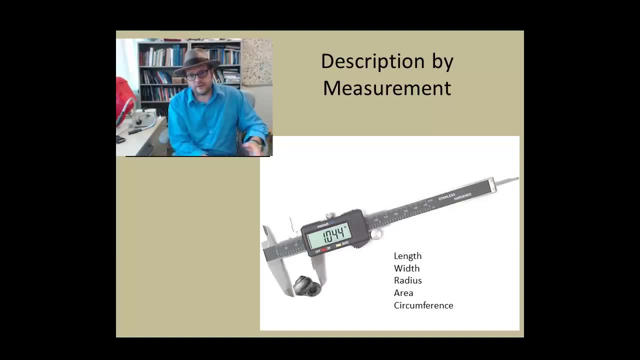 scientists. Descriptive terminology is a pain. We're going to learn a lot of it and go through a lot of these terms, but it's necessary for doing science. The other thing you need to do is take lots of measurements, and I mentioned putting a. 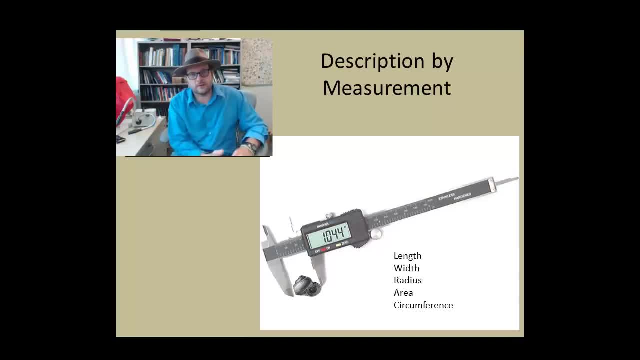 scale bar in your images when you take an image of a fossil. but the other thing you can do is just take lots of measurements: so length, width, the radius, the area, the circumference. A lot of people, a lot of paleontologists, carry around calipers, so whenever they go, 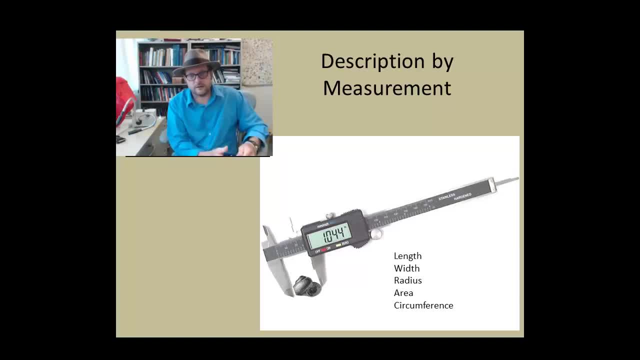 into a museum collection. they can sit down and begin measuring different sizes of things. when collecting data and generating data. One of the fields of science that deals with data collection is data collection. One of the fields of science that deals with data collection is data collection. 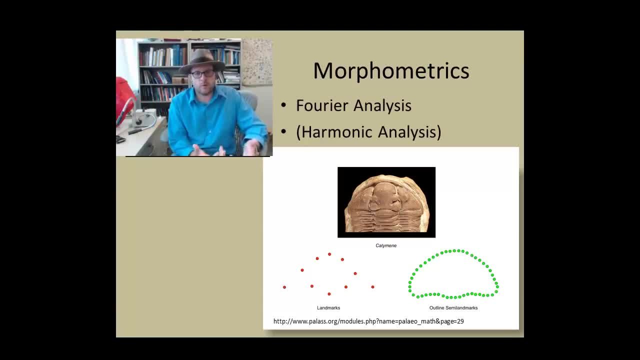 One of the fields of science that deals with data collection is data collection. One of the fields of science that deals with measuring and measuring specimens is morphometrics. Morpho means shape metrics, meaning math or numbers, so it's basically the numbers of shapes. 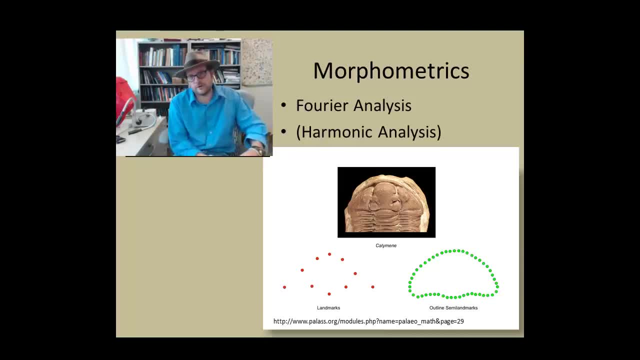 There are different techniques you can do. One of the things I'll talk a little bit about is four-neural analysis, also known as harmonic analysis. For example, what you do is you pick particular landmarks on a specimen that you're comparing and then you can use those landmarks to take measurements. 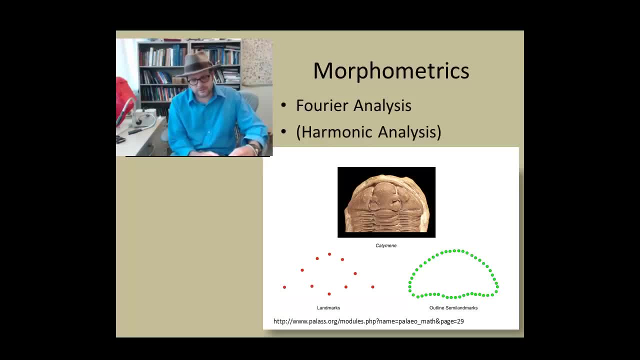 You can take readings in what they call a morpho space, which is basically the three-dimensional space of where those dots occupy. You then can compare that with many, many specimens, and this is called morphometrics. There's lots of science, lots of paleontologists that do this, measuring lots and lots of points. 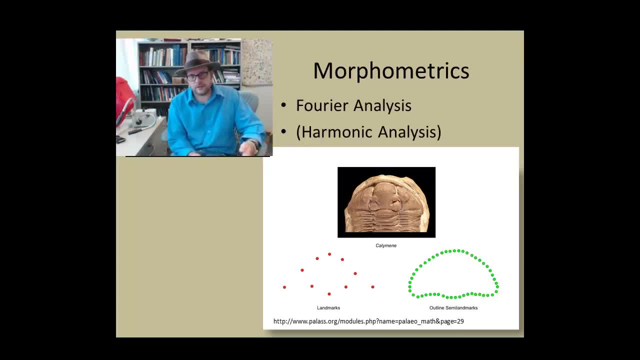 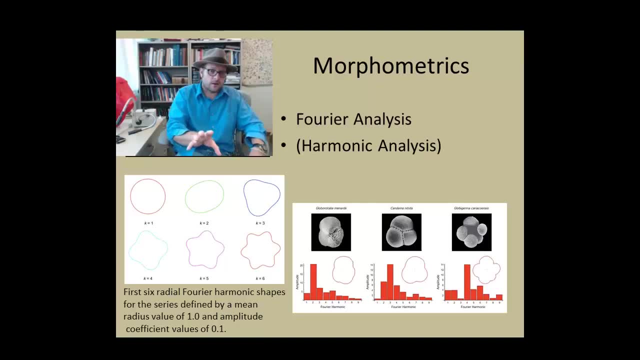 on specimens. Now, this may seem like overkill- you just want to know the length and width and things like that- but sometimes it can be really important, and here's a good example of why you might use four-neural analysis on a bunch of specimens. 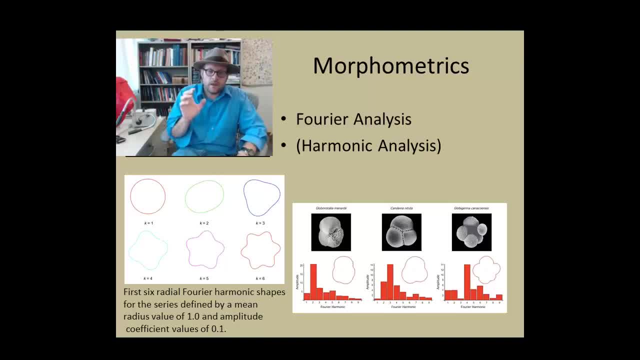 So here we have some forams, and you'll notice that each of these forams that are in this graph here, if you were to measure them, they're basically all the same size. If you measured the circumference, or you measured the width and length, they're all about the 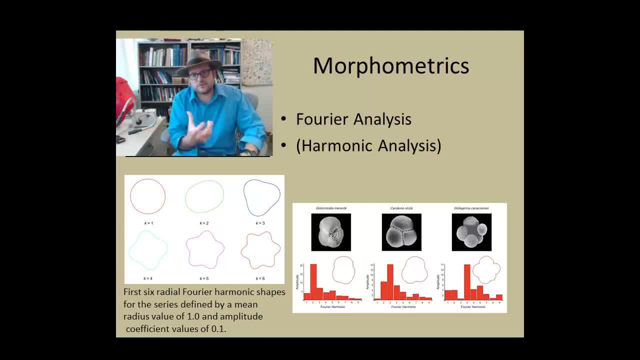 same size, and so they would all group together. However, they have different shapes. One of them is more round and circular, One has these little spheres coming off of it. so one of the things you want to do with morphometrics and analysis like four-neural analysis, is basically outlining those shapes. 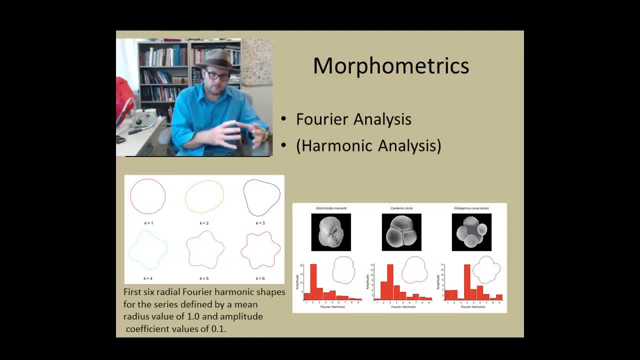 By outlining those shapes you can move from, say, completely a sphere which has a radial analysis of one, so the radius value is one, or you can have one that's very bumpy and have an amplitude that's less than one and be something that's much smaller, like 0.1,. 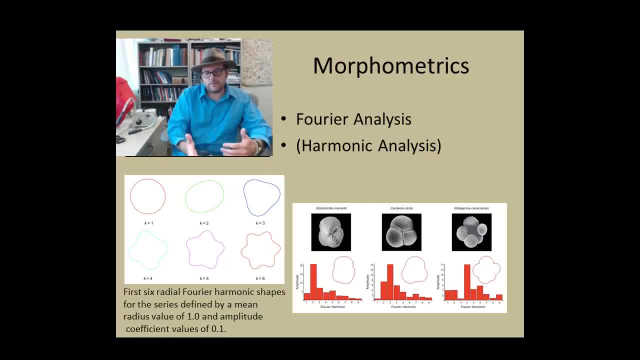 so you have variation in that radius. So these are ways to sort of quantify the bumpiness, using numbers to get at the shape and use this to identify different species or maybe growth series or maybe different dimensions. Oftentimes this is important also to figure out distortion that can happen in the fossil. 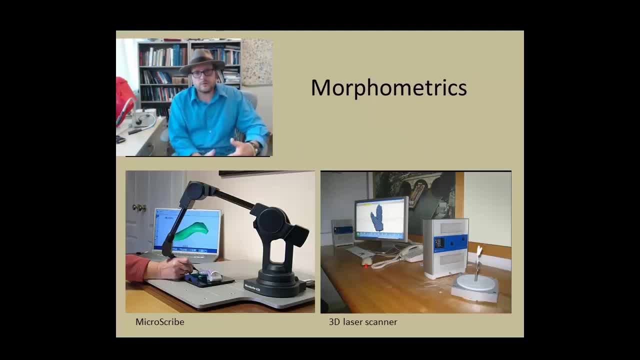 record as well. So there's a lot of tools that you can use to use morphometrics. One of the tools that's often used is what's called morpho. It's called a microscribe, So a microscribe is like this little arm that you attach to a computer and the computer 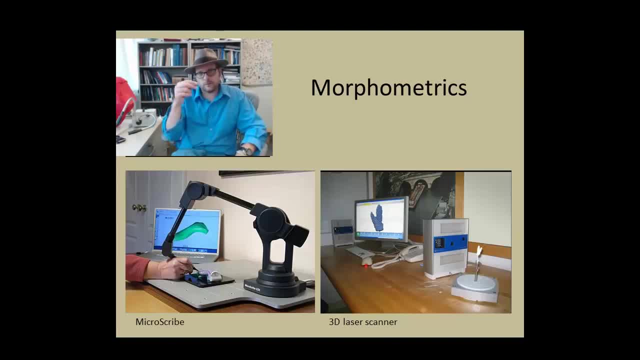 basically records wherever that point of that arm is. He's holding it like a pencil there in that diagram, So a microscribe. he can move that point around the specimen and it records the 3D coordinates, so the x, the y and the z coordinates of those positions as he moves it around the 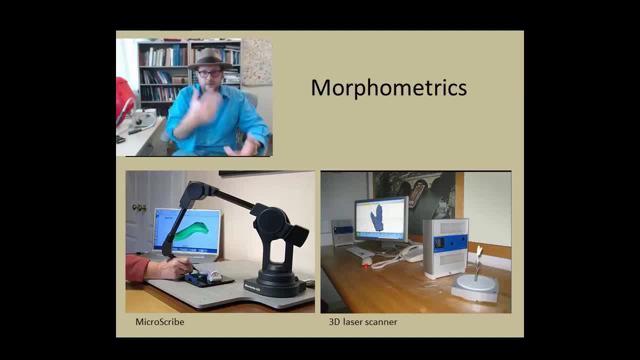 specimen. So then you can take lots of points like this And it captures it into the computer and then it can generate the shape of that fossil. Another thing that's being used more and more is 3D laser scanners. So here we have a fossil that's on a little turntable, and then there's that blue thing. 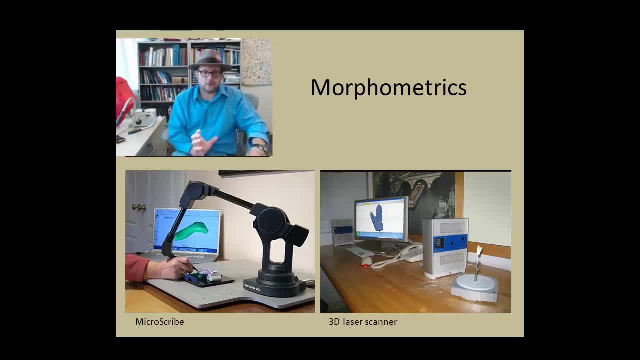 there with the tower, which is actually a scanner, And so the turntable will turn very slowly and the scanner will actually scan the surface of it, And what it's doing is it's sending out the laser beam, It's hitting the specimen and then bouncing back into and registering it. 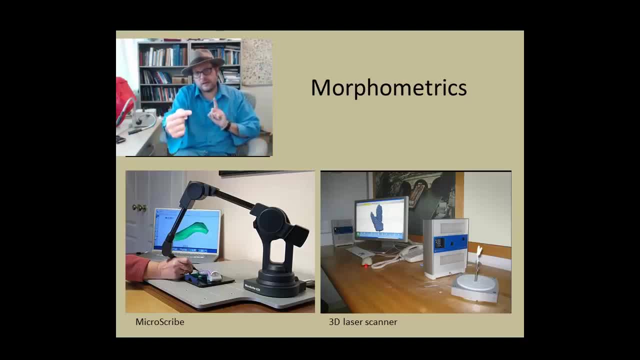 And it registers that distance. So lasers are really good at figuring out the exact, precise distance away. And so then it takes that information, puts it into the computer, as well as the rotation, and you can reconstruct a very nice replica with lots of numbers. 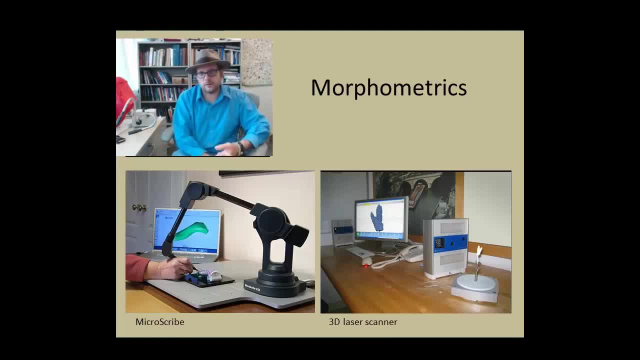 So that's going to be distance numbers to that specimen and reconstruct it in a computer. And it's so easy. It's in a similar fashion, You don't have to hit all the different points. This might be a really good way of capturing some data on something that may be irregular. 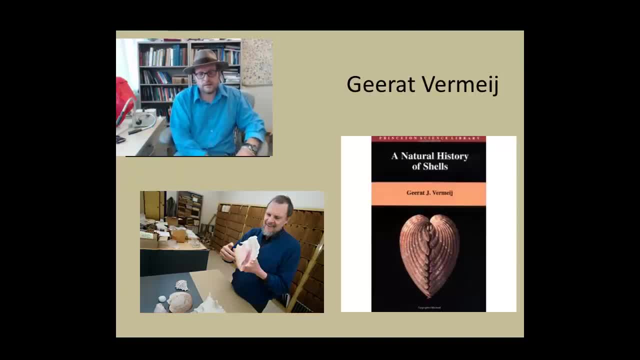 So in this case, it's a fossil coral. Now I've talked about images and the importance of images and taking great images and capturing numbers and all these things, But I wanted to talk a little bit about Girat Vermenghi, who is the world's expert on fossil 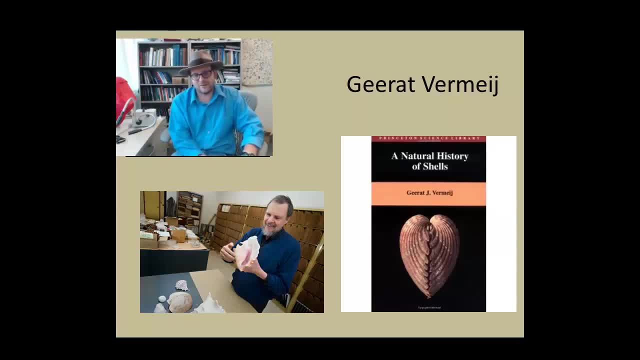 shells. He's published extensively. He's published extensively, In fact. we'll probably read some of his papers. A brilliant scientist has done incredible work on mollusks, published lots of papers. the world's expert on mollusks and he's blind. 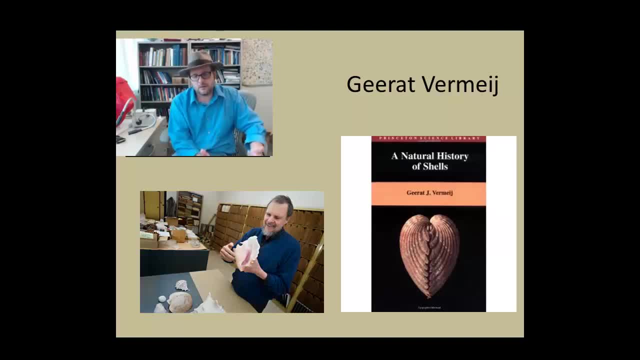 And one of the things that makes him such a great scientist is that he uses his other senses. He uses his hands and feels the different ridges on these fossils, on the textures of the shells, And he's able to encapsulate with his own mind the feeling, the dimensions, the shape. 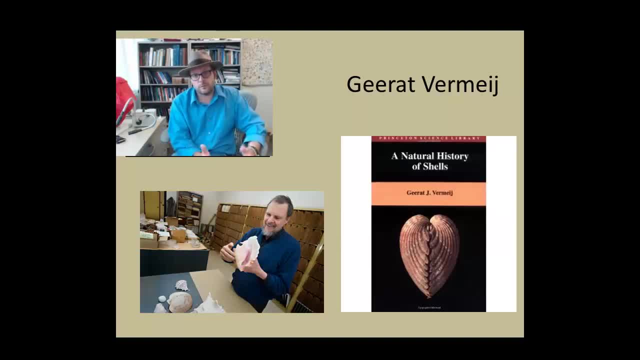 the feel of the fossils, And that allows him to approach fossils in a very different way than many other people who rely on our eyes to see what we're seeing, And I think this is a really good example of how paleontology needs to use all of our 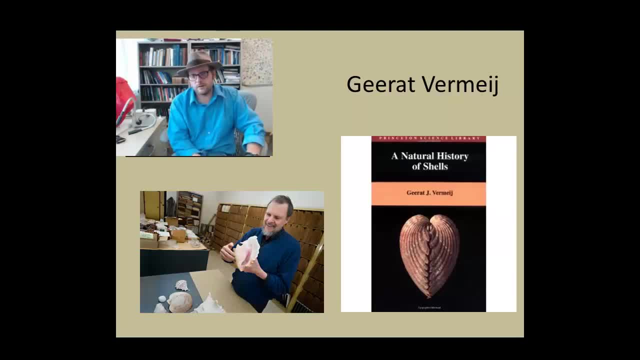 senses when we describe a fossil and a specimen. So you've got a fossil, You've got a fossil, You've got a specimen. You've got a fossil, You've got a specimen. And so even describing the ridges, the roughness, the textures, and reconstructing those things, 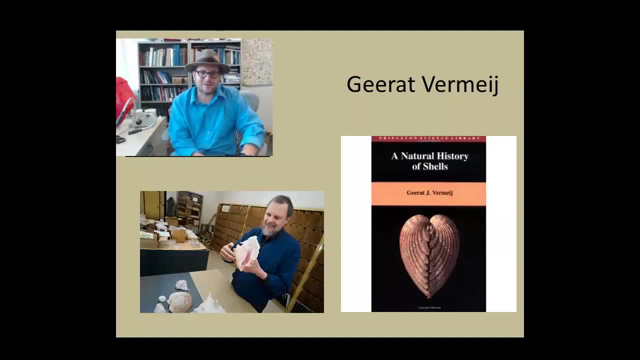 is really important And we shouldn't get bogged down too much on images, So I'll be reading some papers of his, probably when we start covering mollusks, And it's just a really incredible story and he's a great scientist. 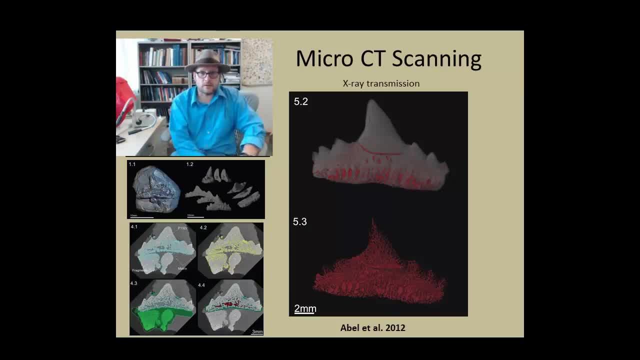 One of the things that's been happening recently is our ability to image the interior portions of fossils and get a view inside fossils, Even taking fossils that are unprepared, putting them into x-rays and basically trying to reconstruct the interior. In the old days you would often times take a fossil and you would put it underneath an 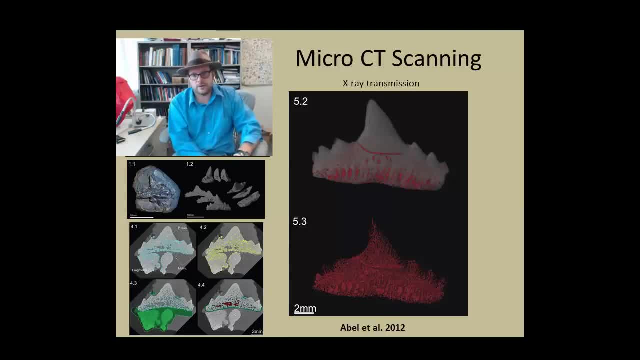 x-ray, shine an x-ray on it And sometimes you could reveal the internal anatomy of the fossil beneath the rock in an x-ray, And that was because of the different densities of the fossil from the matrix around the fossil, And people quickly discovered that you can actually just throw these into a CT scanning. 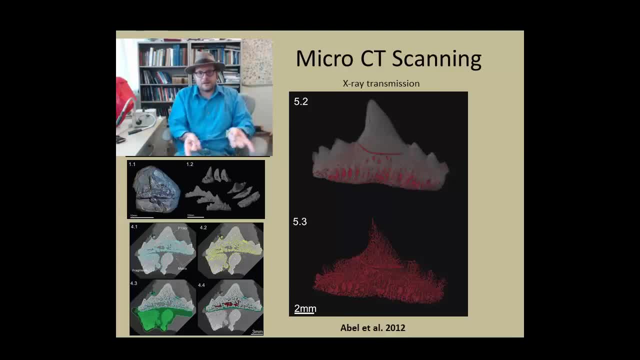 equipment. A CT scanner basically takes x-rays at slices through something, And so CT scanning is often done in the medical profession and takes x-rays of slices, so they can take slices through the body, And people started throwing fossils onto CT scans and getting these slices. 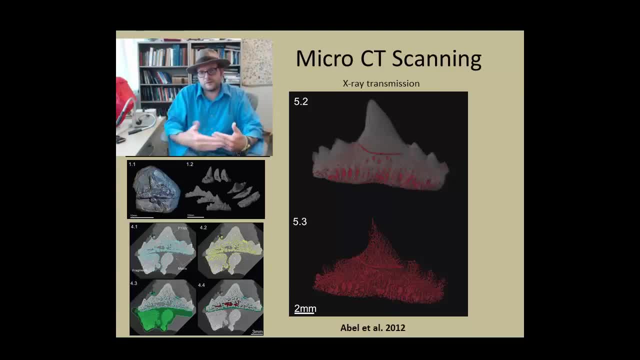 You could take these slices, these x-ray slices. You could take these x-rays And then stitch them together to create a 3D image. But you can also go in and look at the interior structure inside the fossils. In the last few- probably 15 years, micro CT scanning has become a new tool. 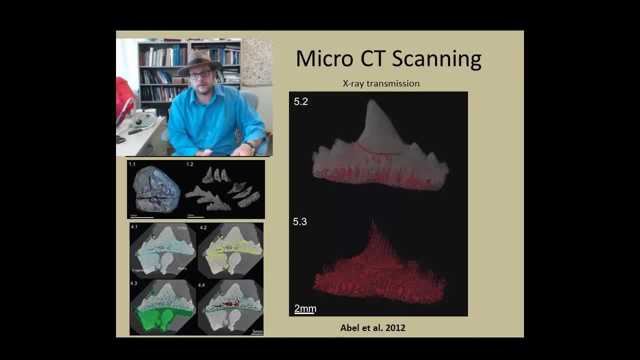 Micro CT scanning is a little bit than traditional CT scanning in that it's much smaller, So they can do very small specimens. So in the old days you could do this with dinosaurs, maybe some large mammal fossils, things like that, That were human size.